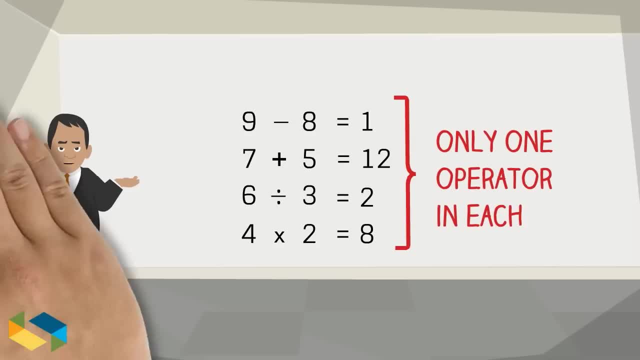 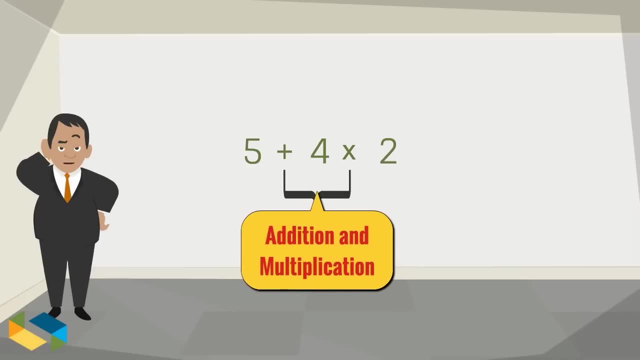 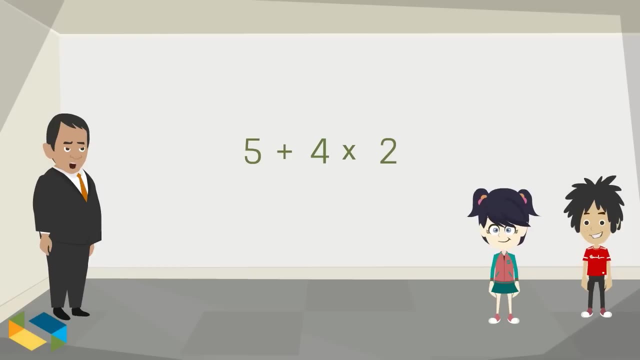 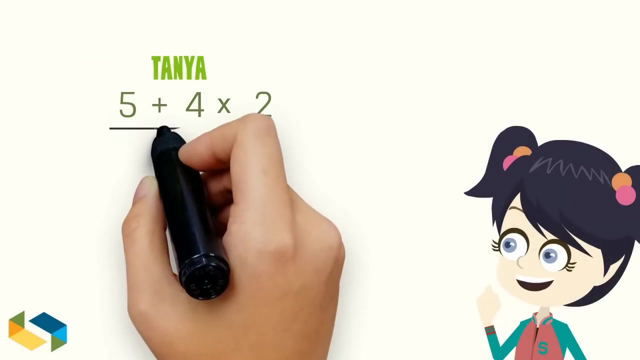 is only a single operator involved in each. But when we have expressions like these, where multiple operators are involved, things could get a little trickier. So by giving this same expression separately to both of you to solve, you go first Tanya. 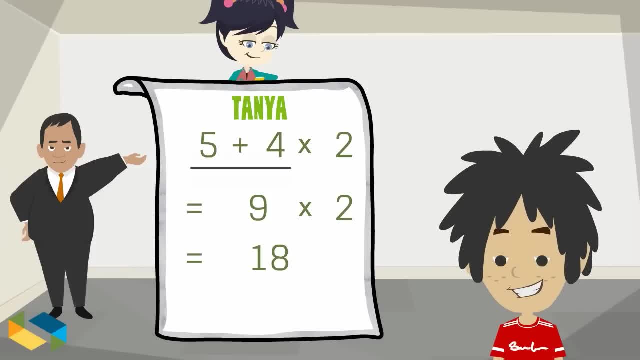 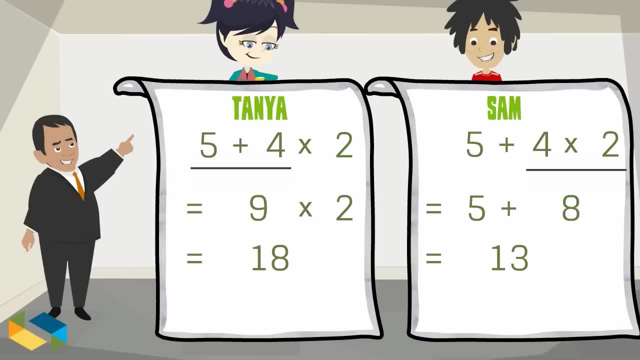 Your turn now, Sam. Tanya's turn. Tanya, I'm going first. Oh, no, Tanya's going first, I'm going first, I'm going first, I'm going first. Both Tanya and Sam have got different answers. 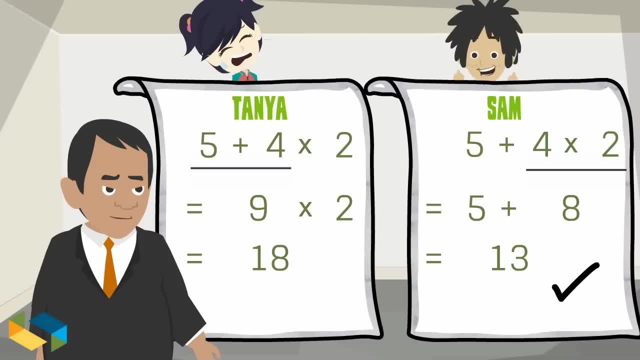 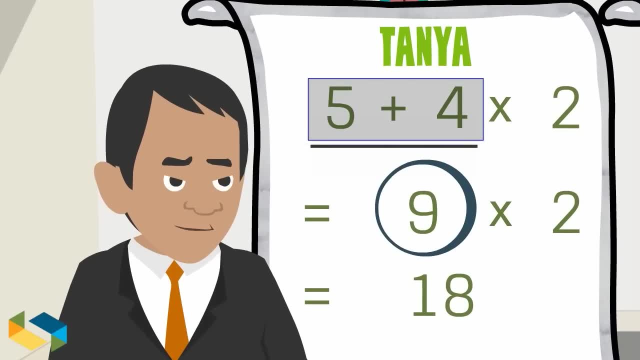 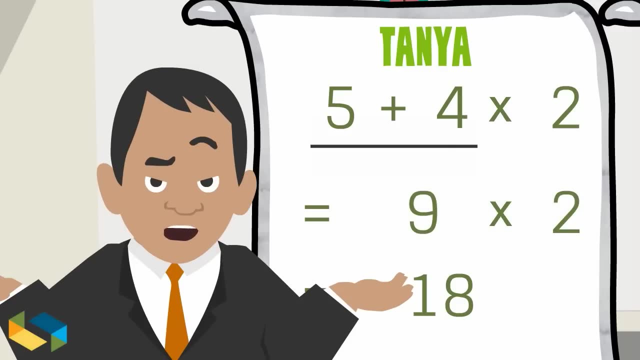 But the correct answer is 13.. Let's find out where Tanya went wrong. She got 5 plus 4, which is 9.. That is correct, And 9 times 2 is 18.. That is also correct. So where did she go wrong? 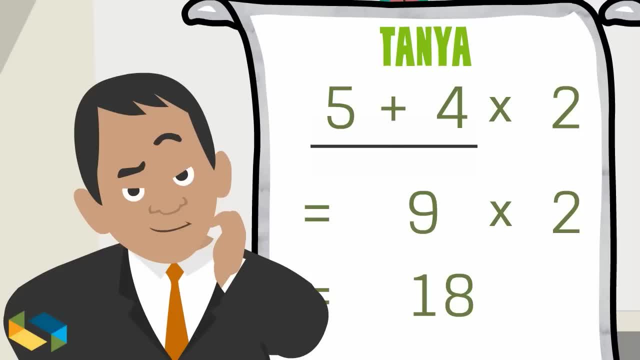 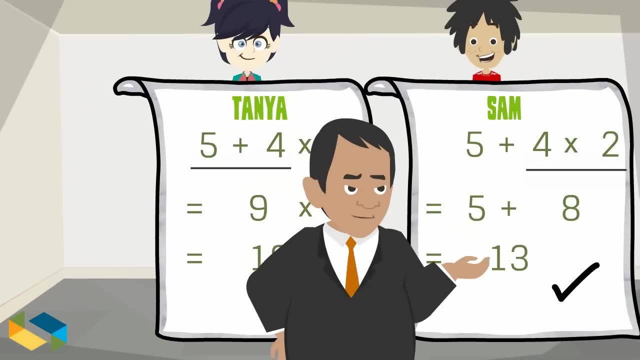 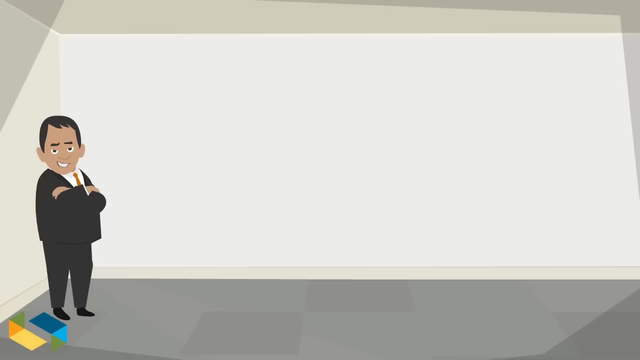 Well, the problem lies in the order she did these operations. She did the addition first, followed by the multiplication, whereas it should have been the other way round. You may be wondering: how do we know what operation comes first and what comes next? 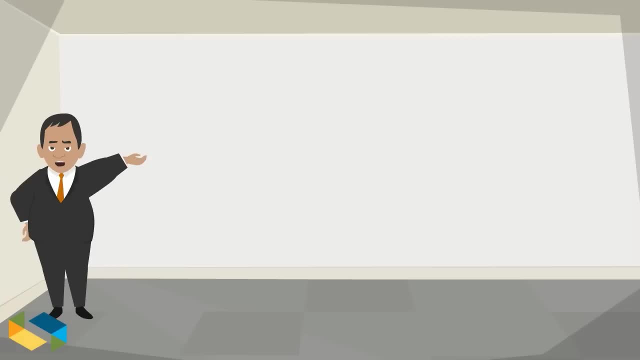 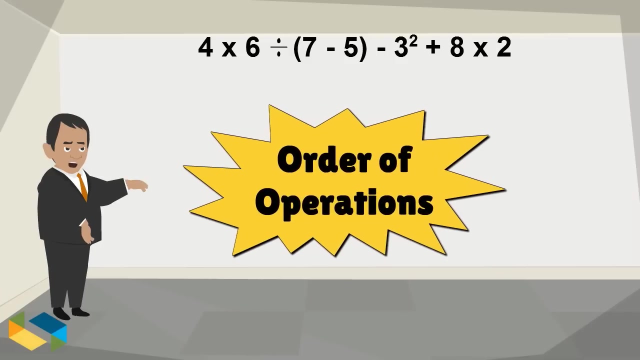 Well, there are steps you have to remember and follow in a sequence called the order of operations. Let's learn this rule through this example. This problem may look complicated, but if you just stick to the sequence or order of doing the operations, it turns out to be very simple. 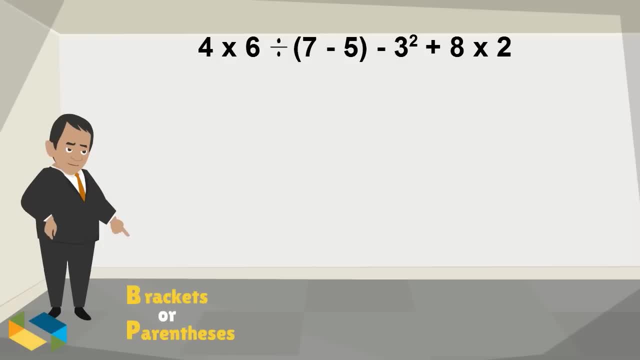 Let's have a look. The first thing you always look to solve are brackets or parenthesis. So for now we ignore the rest of the problem and focus only on solving what's inside the brackets. 7 minus 5 is 2 and our first step is done. 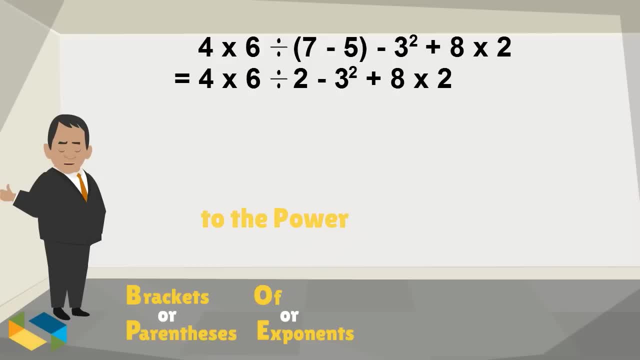 Next we look for any exponent or power in the expression. We have here 2.. We have here 3 to the power of 2 or 3 squared, and that's what we solve as the next step. In the next step we pick the division and multiplication together, but solving them. 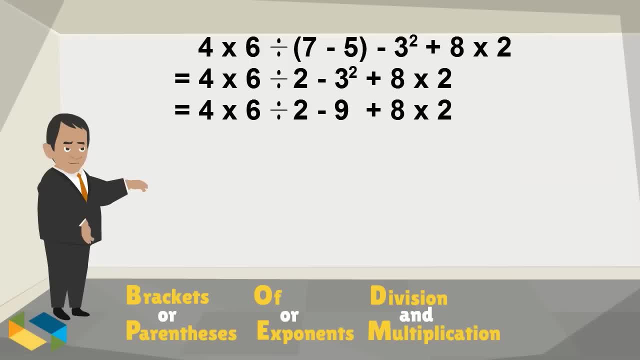 one by one as we go from left to right, 4 times 6,, as you see, is the first of the division or multiplication operations. starting from the left, We get the product 24, which we now have to divide by 2.. 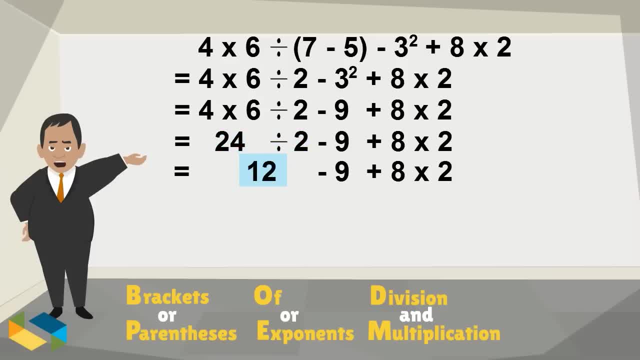 As this is the next operation in line, We write down the answer as 12, retaining the rest of the problem as is. As we proceed to the right, we skip these addition and subtraction parts, as there is still a multiplication operation left to perform, which is 8 times 2, and this gives us 16.. 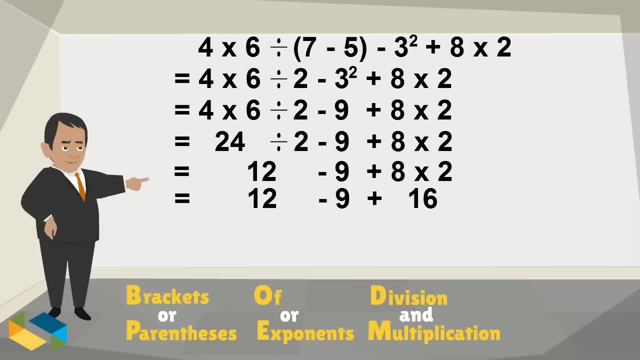 Now you see, we have completed all the division and multiplication operations and are left with only the addition and subtraction ones. We solve these together as we proceed to the next step. We have now completed all the division and multiplication operations and are left with only the addition and subtraction ones. 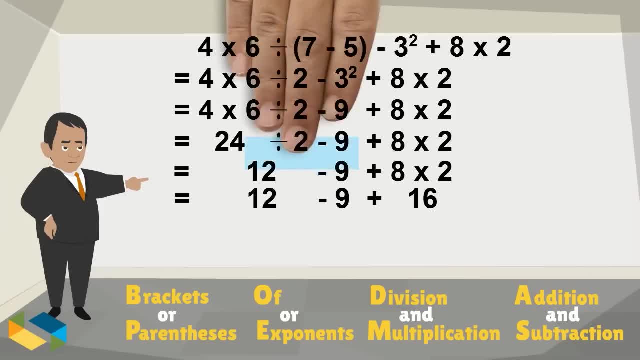 Then we just have to work on the addition and subtraction part as we proceed from left to right. So we have 12 minus 9, which is 3, and this leaves us with 3 plus 16, giving us 19 as our answer to the problem. 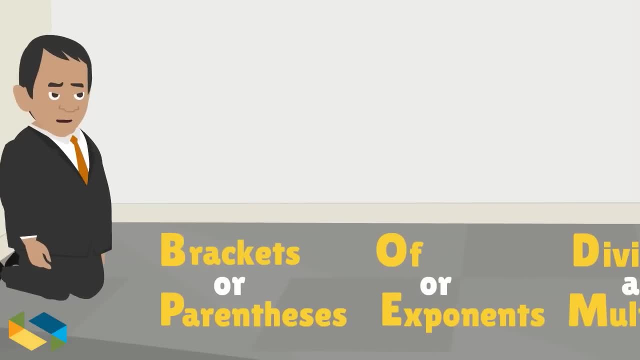 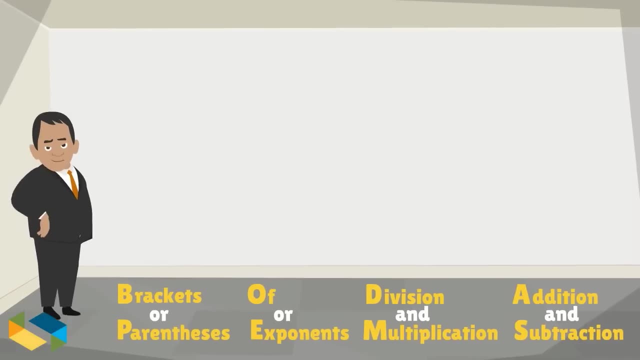 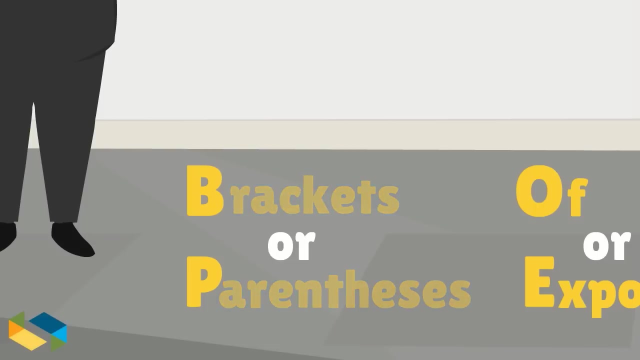 Simple, wasn't it? So if you remember this sequence of steps and just stick to it, you will never fail in getting the right answer. Now, to make things easier, we will devise a quick way to recollect this sequence of steps. For the brackets or parenthesis, we use B or a, P. 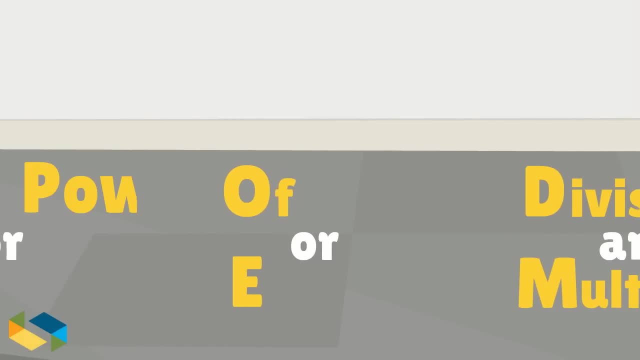 For exponents, we can use E. We can also use the letter O, as in the off, for depicting the exponents. Next, we simply use M and D for multiplication and division respectively. The order of letters M and D is not important. 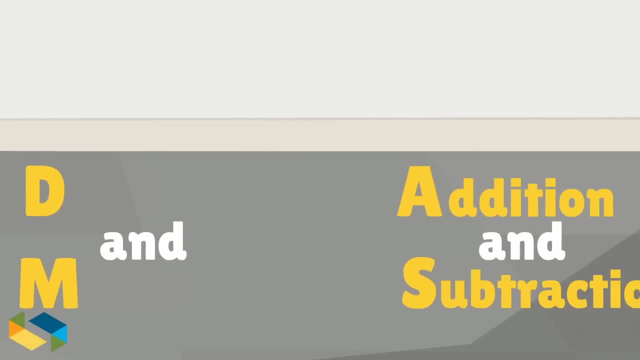 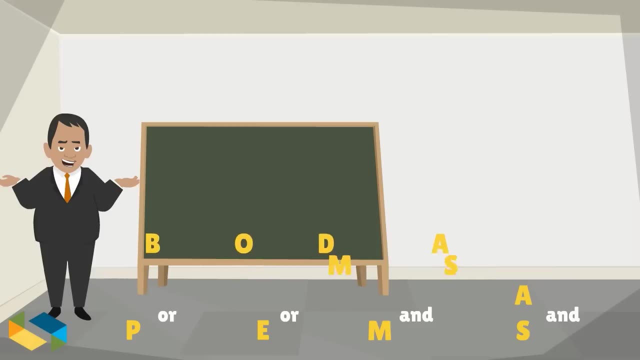 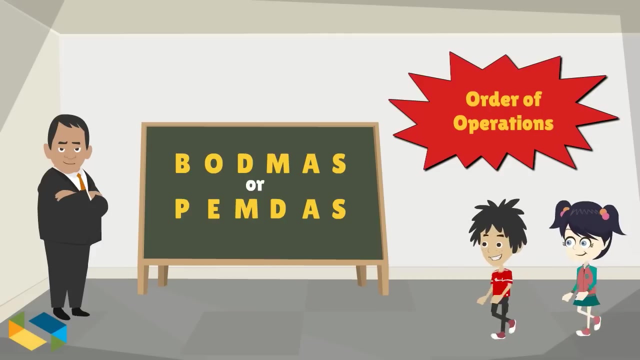 Just remember that these have to be done before the addition and subtraction which we depict with the letters A and S. So there you have it. We have Bodmas or Pemdas as short words to remember the order of operations. So, kids, happy practicing to you.